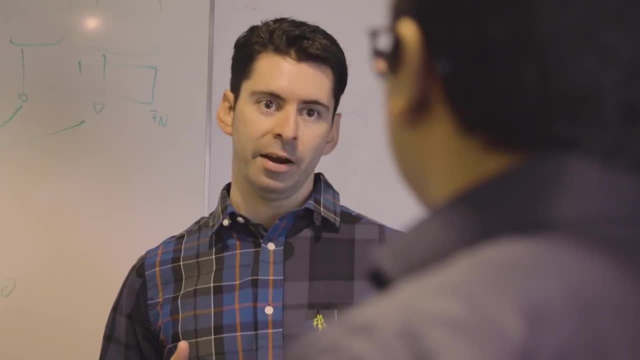 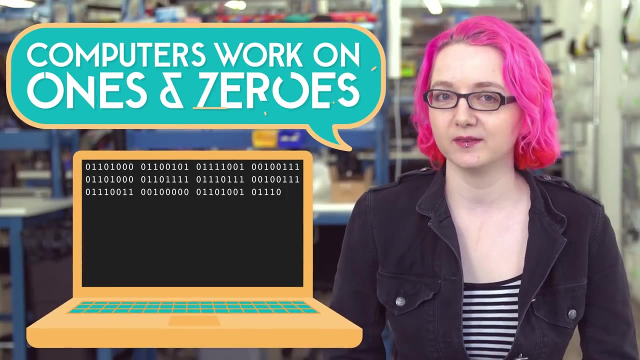 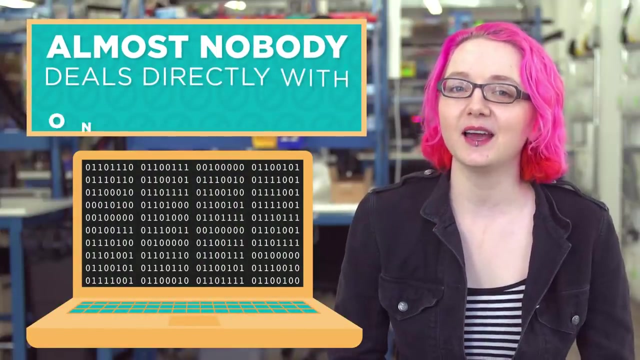 technology to help us solve some of the big social problems of our times. You may have heard that computers work on ones and zeros, or you may have seen scary looking visuals like this, but almost nobody today actually deals directly with these ones and zeros, But ones. 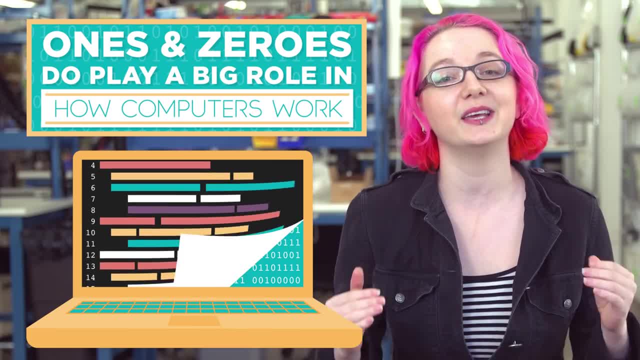 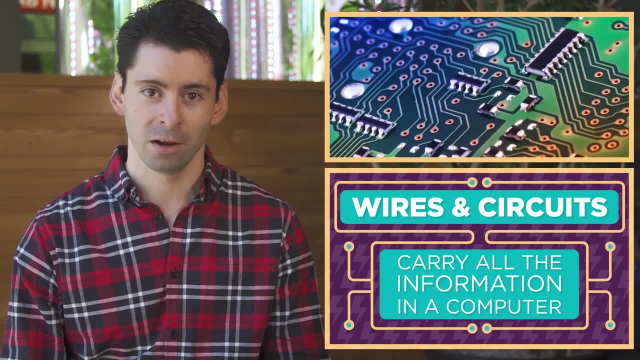 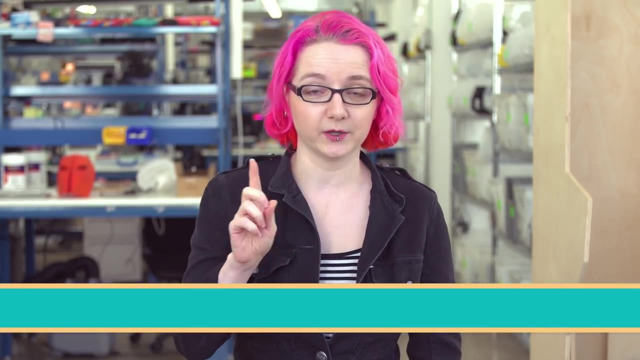 and zeros do play a big role in how computers work. on the inside, Inside a computer are electric wires and circuits that carry all the information in a computer. How do you store or represent information using electricity? Well, if you have a single wire with electricity flowing through it. 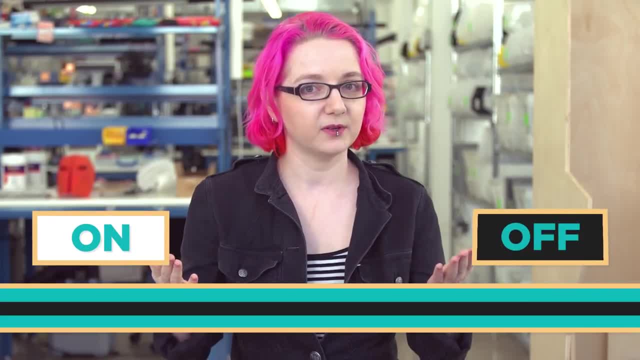 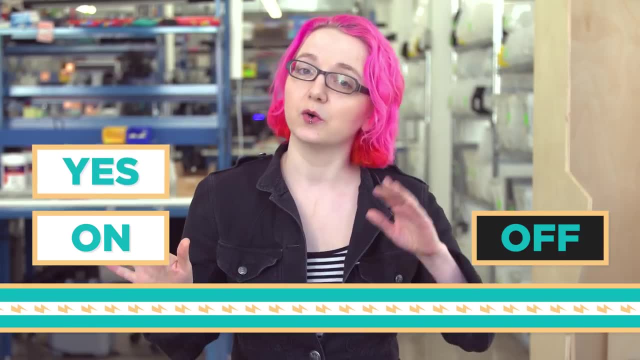 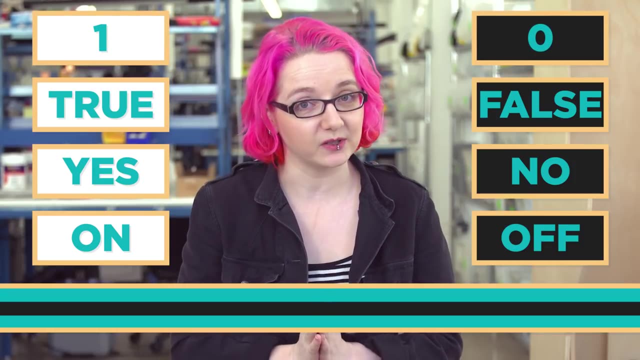 the signal can either be on or off. That's not a lot of choices, but it's a really important start. With one wire we can represent a yes or no, true or false, a one or a zero or anything else. with this on off state of a single wire is called a bit, and it's the smallest piece of information. a. 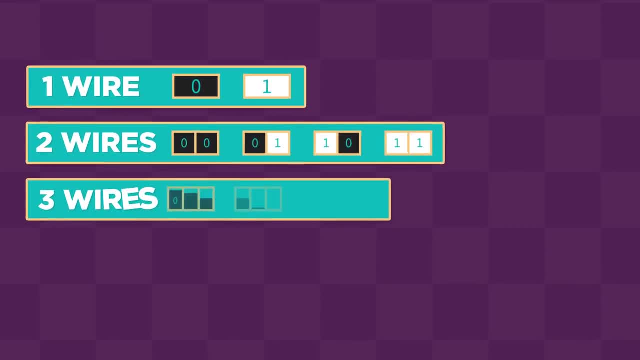 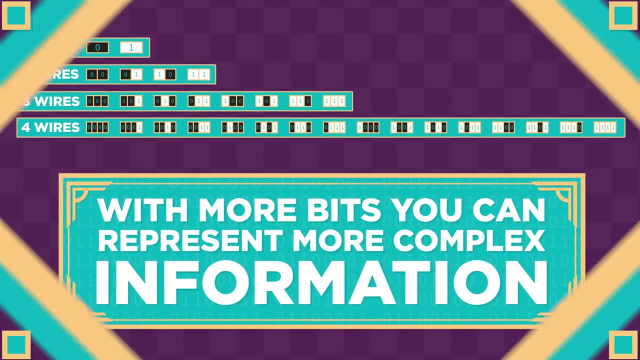 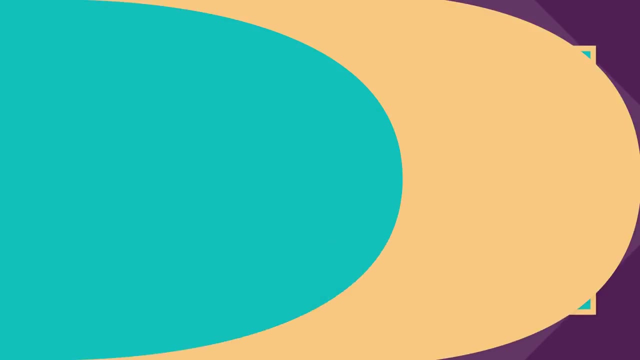 computer can store. If you use more wires you get more bits, more ones and zeros. with more bits you can represent more complex information. But to understand that we need to learn about something called the binary number system. In the decimal number system we have 10 digits, from 0 to 9, and 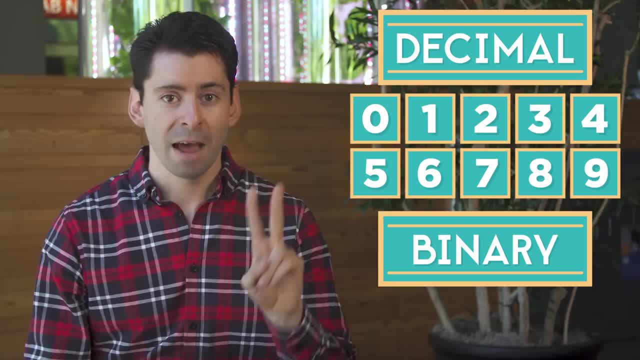 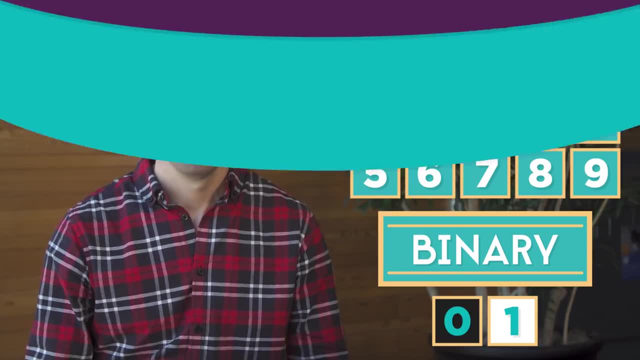 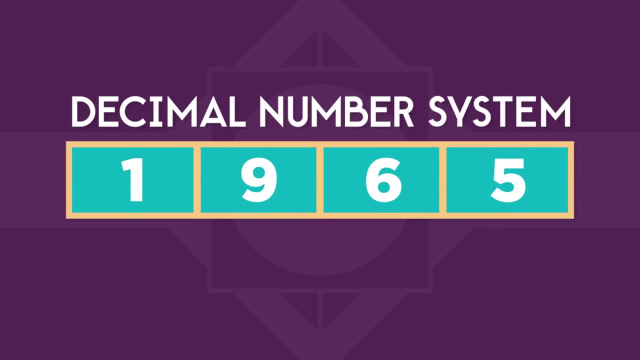 count. In the binary number system we only have two digits: 0 and 1.. With these two digits we can count up to any number. Here's how this works In the decimal number system we're all used to. each position in a number has a different value. There's the one position, the 10 position. 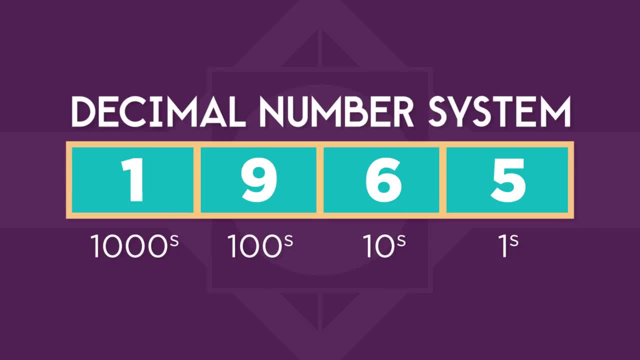 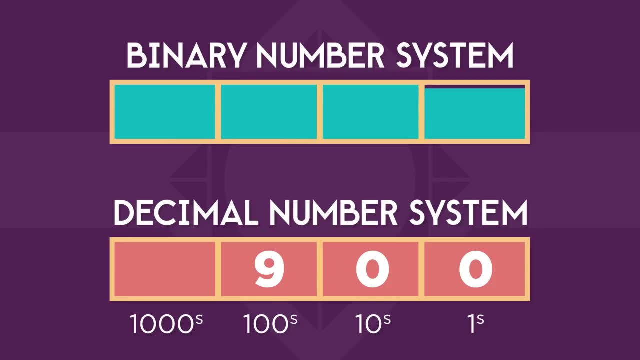 the 100 position, and so on. For example, a 9 in the 100 position is a 900.. In binary, each position also carries a value, but instead of multiplying by 10 each time we multiply by 2.. So there's the 1's position, the 2's position, the 4's position. 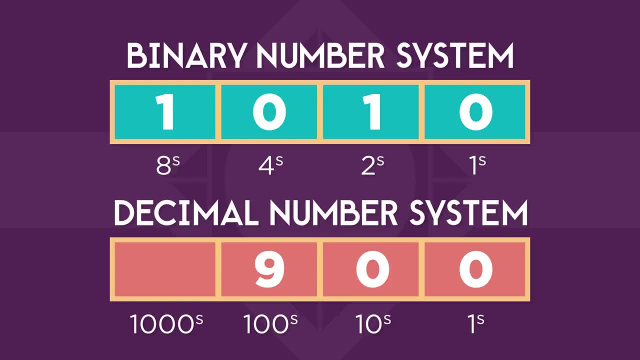 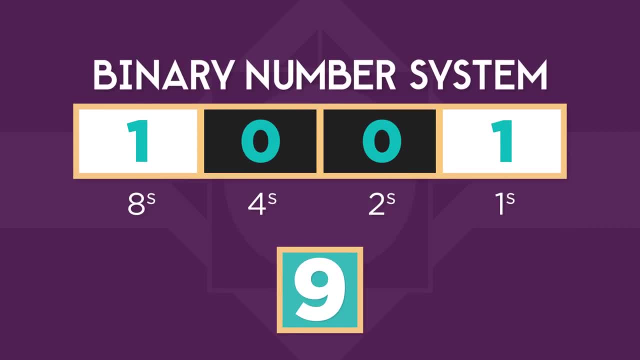 the 8's position and so on. For example, the number 9 in binary is 1 0 0, 1.. To calculate the value, we add 1 times 8 plus 0 times 4 plus 0 times 2 plus 1 times 1.. 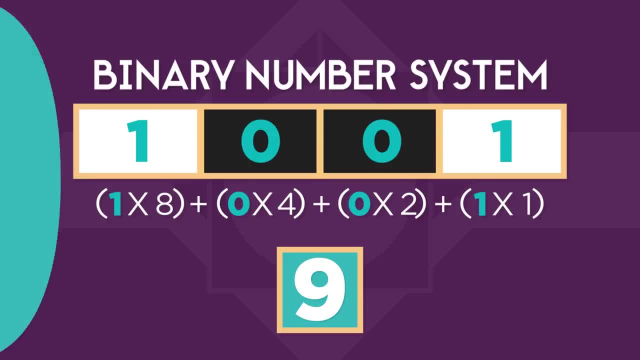 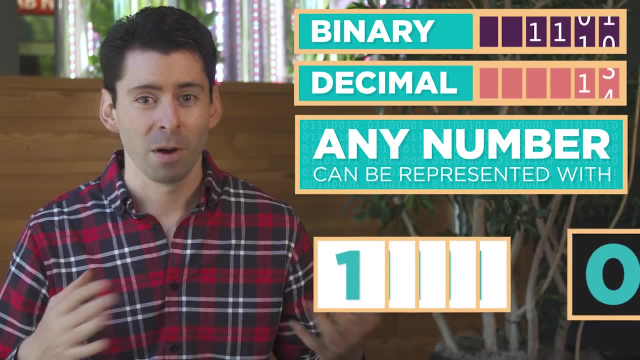 Almost nobody does this math, because computers do it for us. What's important is that any number can be represented with only 1's and 0's, or by a bunch of wires that are on or off. The more wires you use, the larger the numbers you can store. 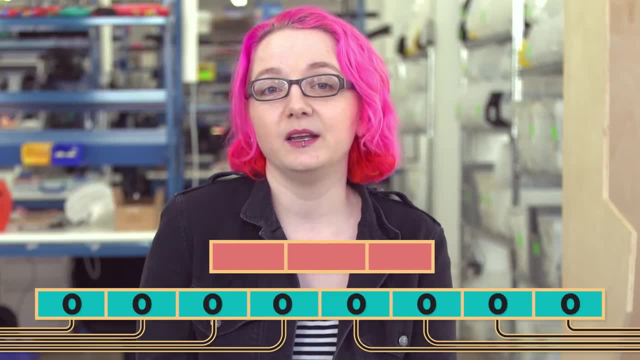 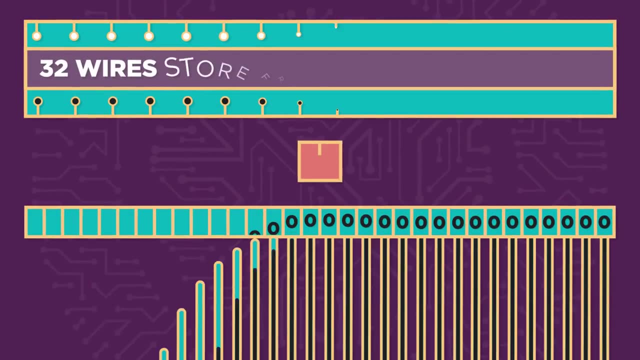 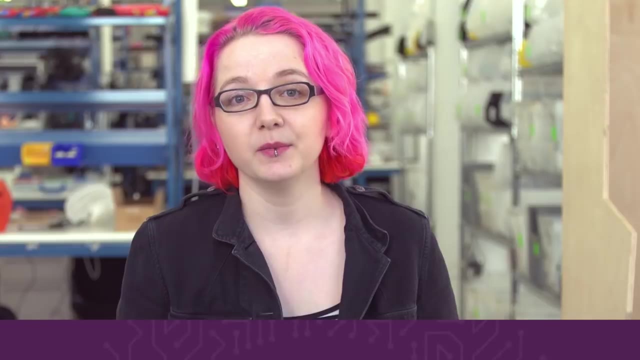 With 8 wires, you can store numbers between 0 and 255.. That's 8: 1's. With just 32 wires, you can store all the way from 0 4 billion. Using the binary number system, you can represent any number you like. 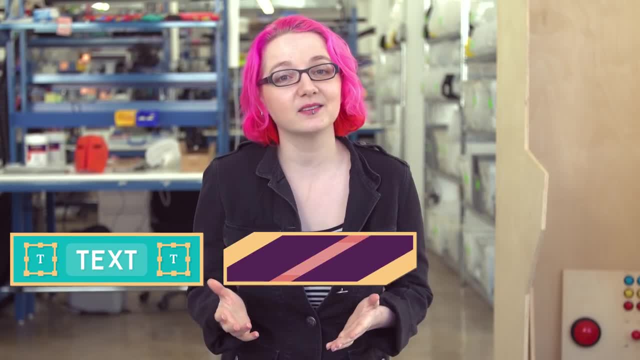 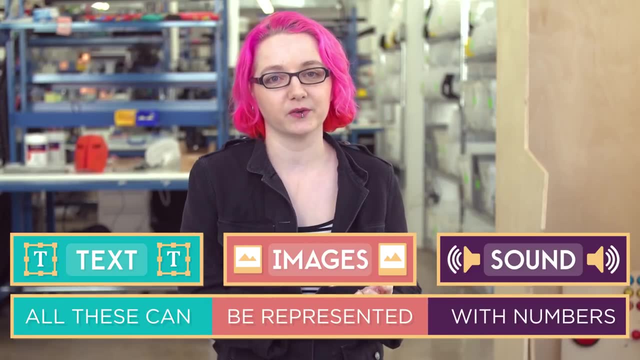 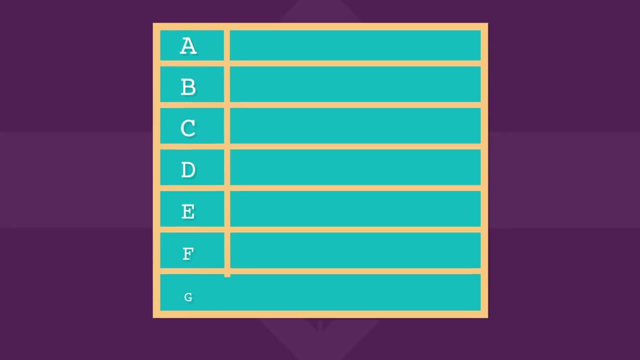 But what about other types of information like text, images or sound? It turns out that all these things can also be represented with numbers. Think of all the letters in the alphabet. You could assign a number to each letter: A could be one, B could be two, and so on. 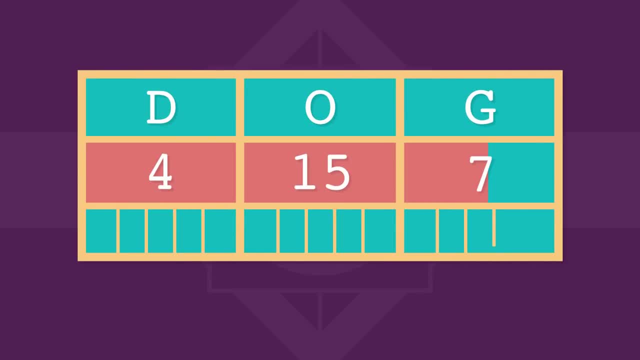 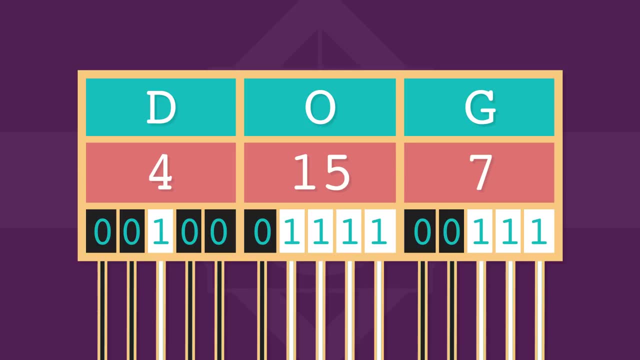 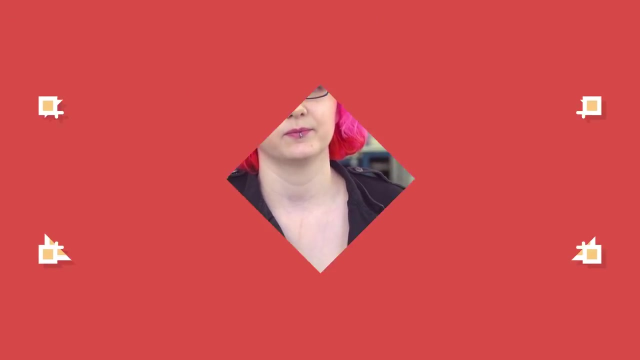 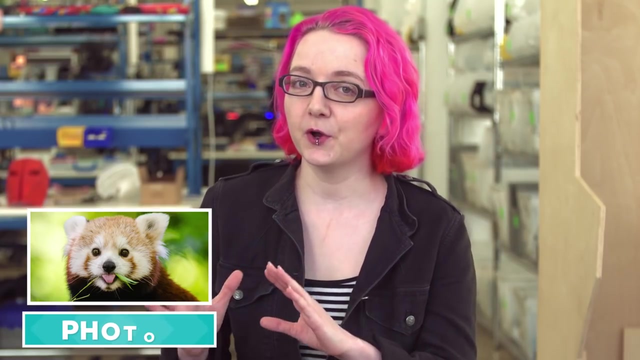 You can then represent any word or paragraph as a sequence of numbers And, as we saw, these numbers can be stored as on or off electrical signals. Every word you see on every web page on your phone is represented using a system like this. Now let's consider photos, videos and all. 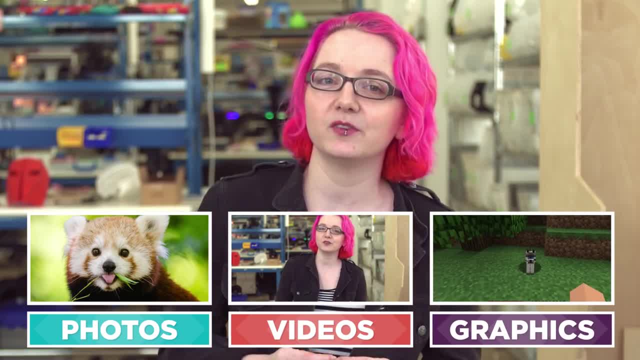 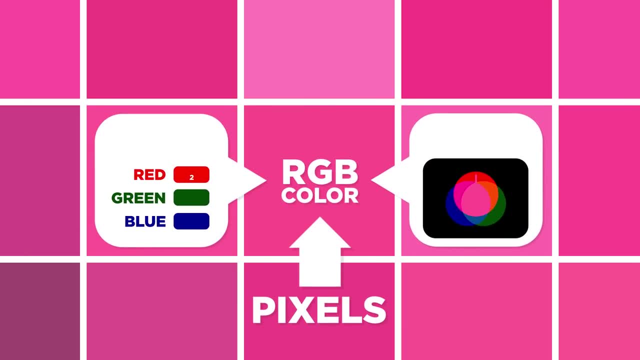 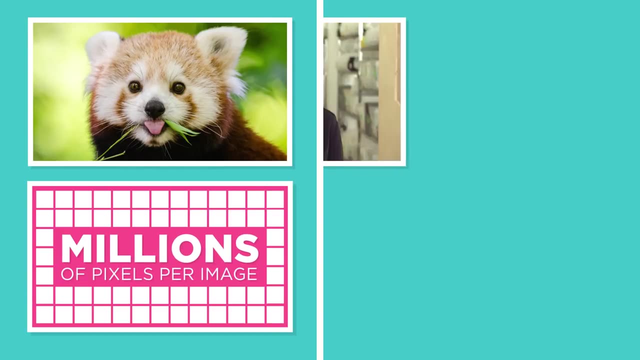 the graphics you can use to represent a number. All of these images are made out of tiny dots called pixels, And each pixel has a color. Each of the colors can be represented with numbers. When you consider that a typical image has millions of these pixels and a typical video. 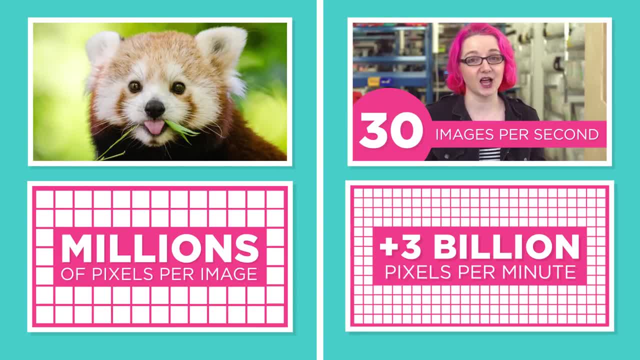 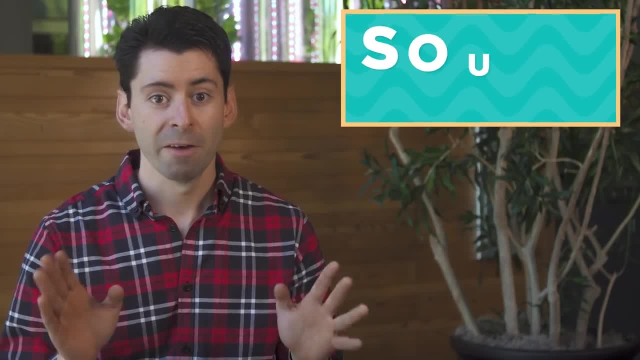 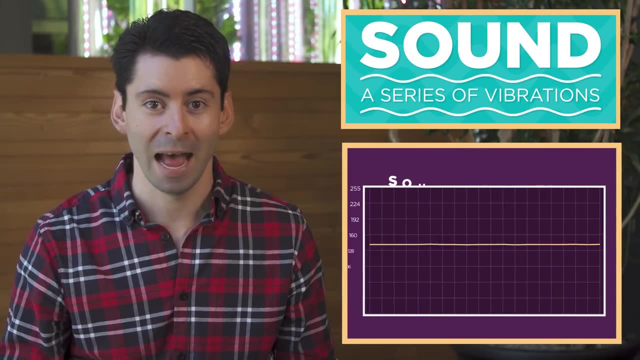 shows 30 images per second. we're talking about a lot of data here. Every sound is basically a series of vibrations in the air. Vibrations can be represented graphically as a waveform. Any point on this waveform can be represented by a number. 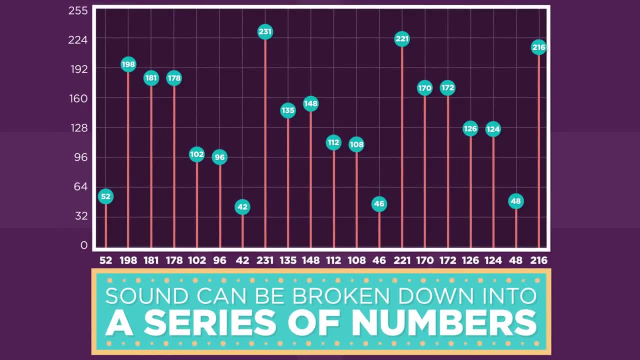 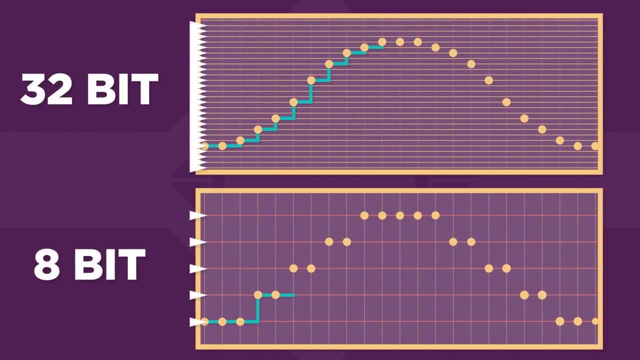 And this way any sound can be broken down into a series of numbers. If you want higher quality sound, you would pick 32-bit audio over 8-bit audio. More bits means a higher range of numbers. When you use a computer to write code, you need to know how many pixels you have.